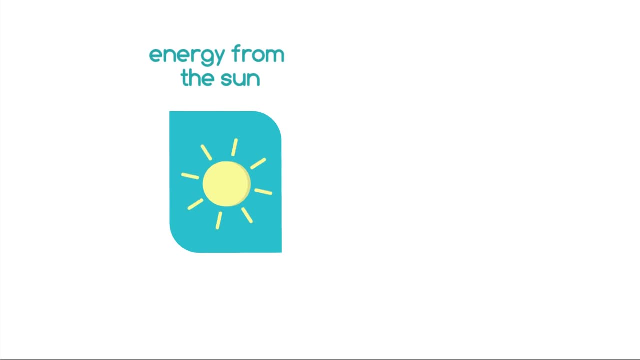 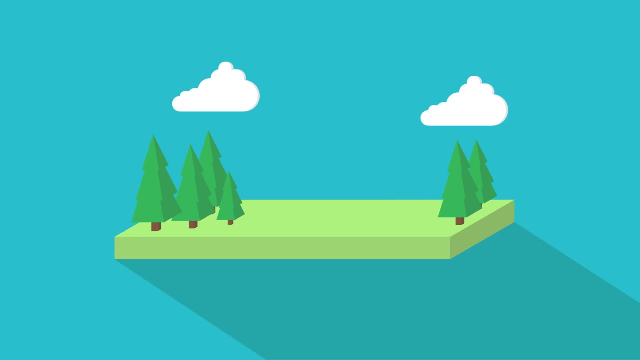 in nature, again using energy from the sun, and we will also see the part played by mankind when we use fossil fuels. First of all, the natural carbon cycle. Can you remember what the process is called where plants capture carbon and give off oxygen? 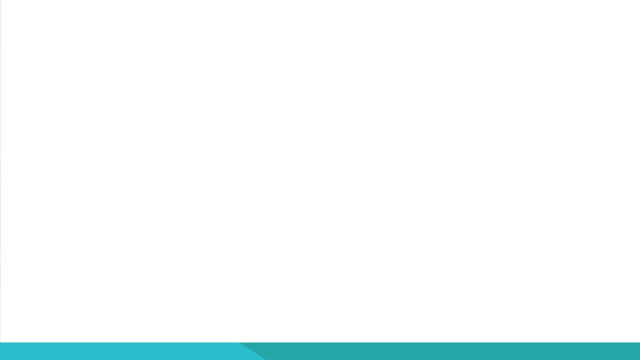 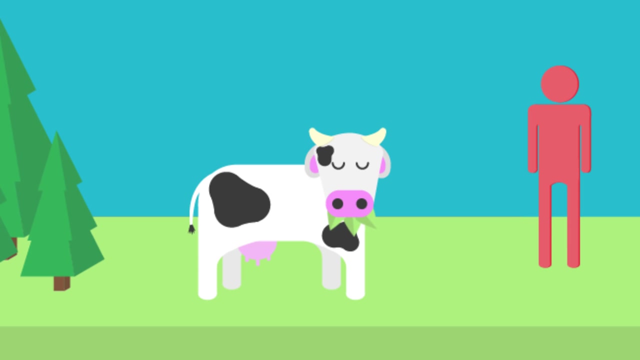 Pause the video whilst you think. Did you remember that this process is called photosynthesis? The carbon is used to build up new plant material. Animals eat the plants or other animals to build up their bodies, To obtain energy. for all these living processes, plants and animals take in oxygen. 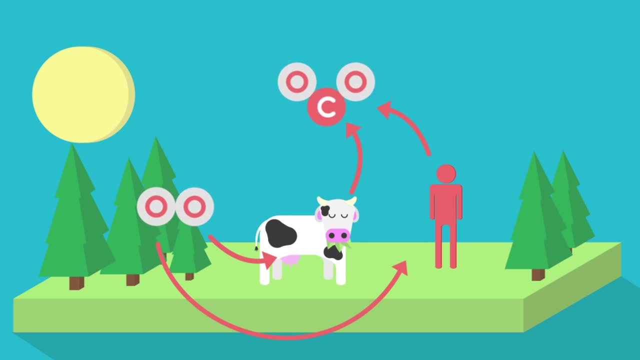 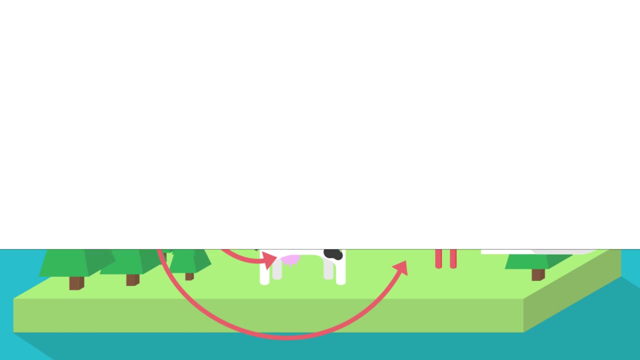 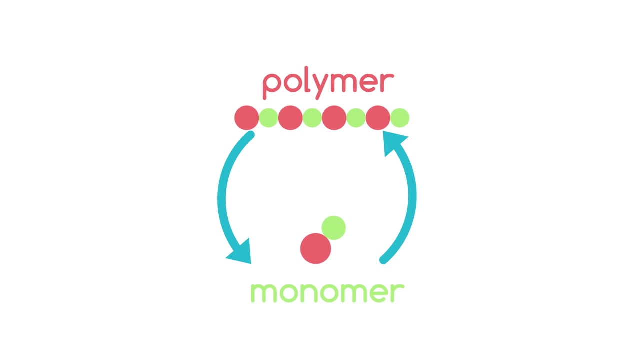 And re-join it with the carbohydrates, so returning the carbon dioxide to the atmosphere. Do you remember what this process is called? Pause the video. This process is called respiration. Now let's put some details into this. As they grow, all living things have to build up large polymer molecules from small molecules. 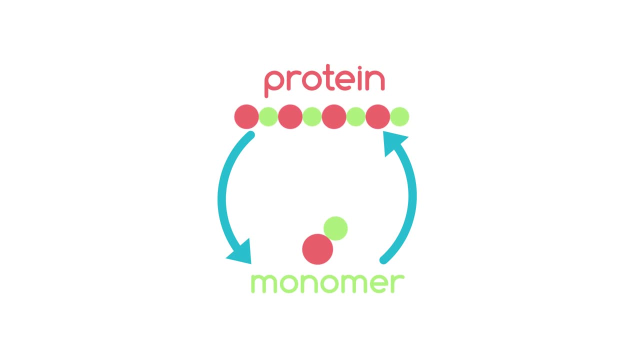 Protein, for example, to make your skin and muscles And other organs. comes from joining amino acids together, Cellulose and starch to make the leaves, flowers, trunks, roots and all parts of plants. From joining sugars and DNA to make the genes which control living things from the 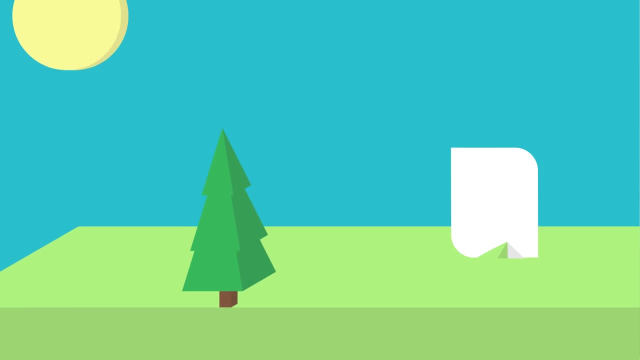 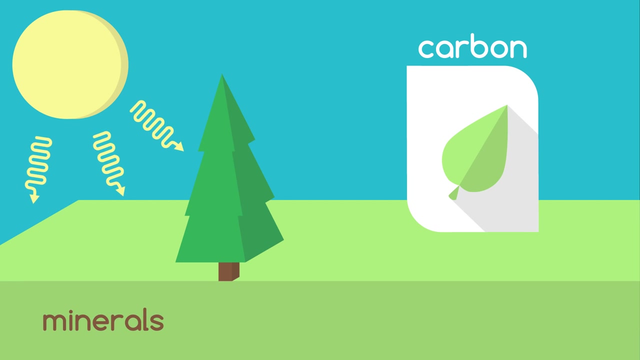 bases and the sugar and phosphate. Plants can make these simple molecules from the carbon they capture from photosynthesis, with added elements from the minerals they get from the cells. This process is called respiration. This process is called respiration. This process is called respiration. 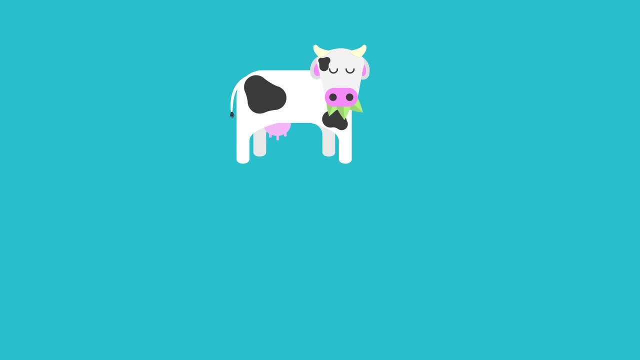 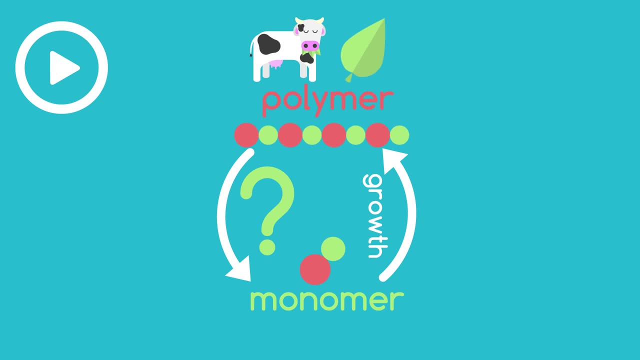 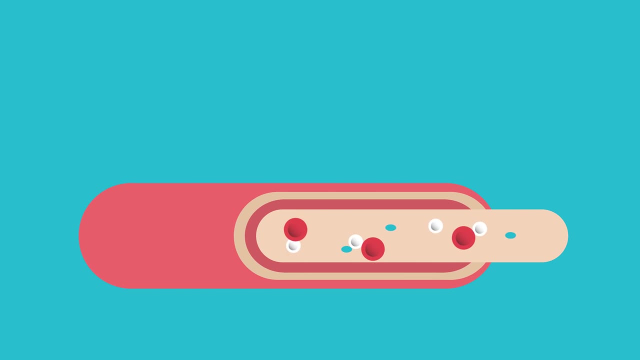 Do you know what? this process is called Pause, whilst you think of an answer? This is called digestion: breaking the food into little bits so it can get into our blood. All of this, of course, needs lots of energy, And living things get their energy from respiration.